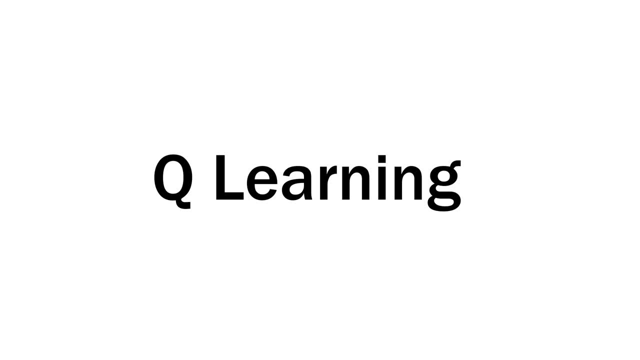 Hello everyone. Today marks the start of a new tutorial series I'm doing on Q-Learning. Here we will explain it and, if you're interested, definitely check out the follow-up videos for in-depth tutorials. Q-Learning is a type of reinforcement learning, If you know, of supervised 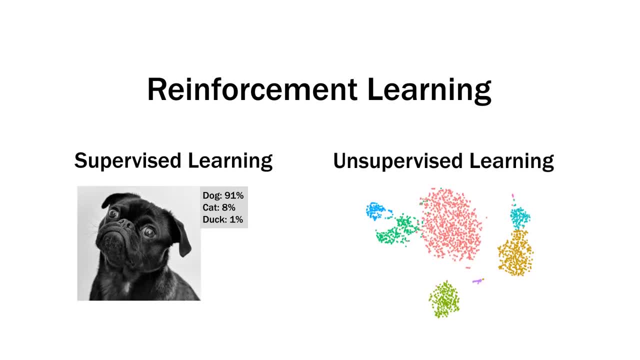 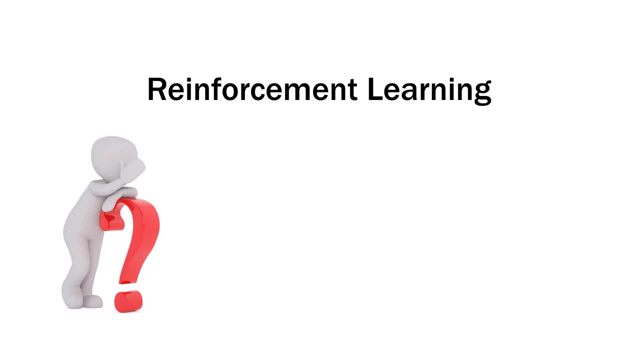 learning or unsupervised learning. reinforcement learning is a whole other paradigm that sits alongside of those. So what is it? Well, it is a way to solve a set of problems where you are trying to maximize some reward. Now, that's the technical mumbo jumbo. but what about an actual? 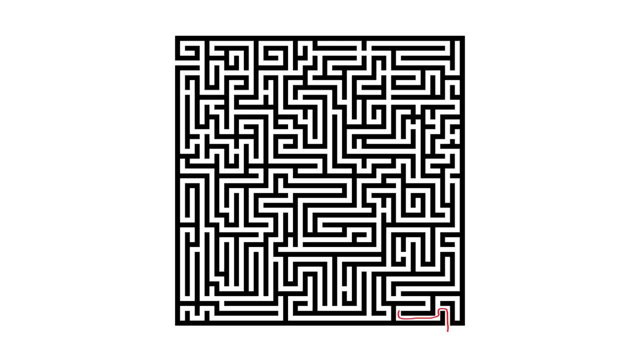 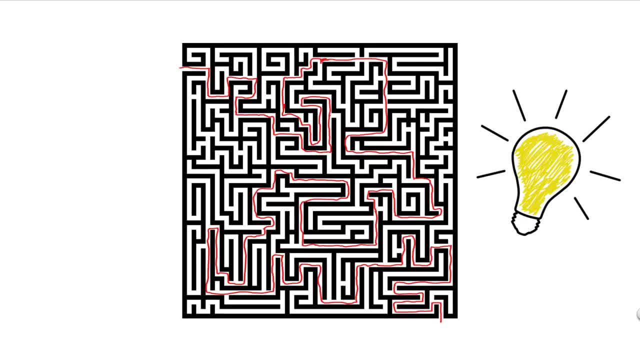 example, Say, we want to solve a problem and although we might not know exactly how to solve it a lot of the time we can at least judge how good a solution is. Those are the types of problems that reinforcement learning is trying to solve. 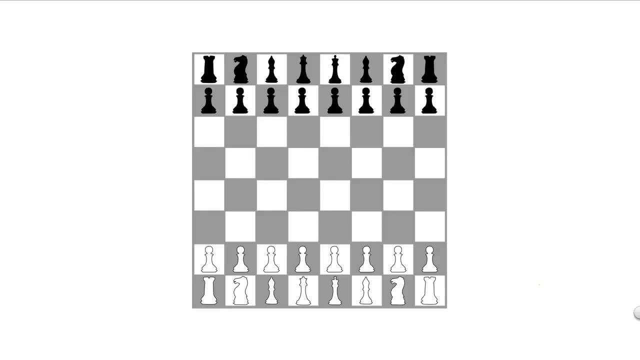 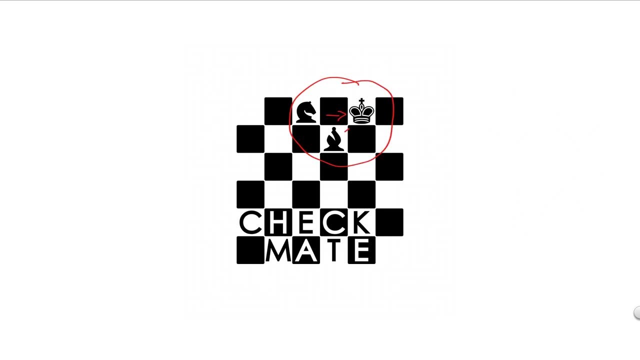 So let's look at a few Q-Learning Backflips. First we can look at chess players. It's very easy to tell when a game is won or lost, sometimes even before it happens, but it's very difficult to make up an actual strategy to win. 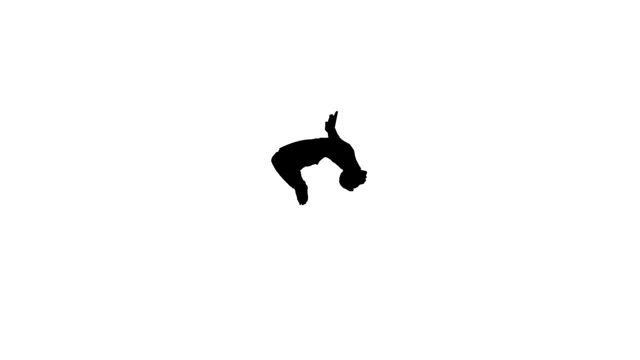 Or think of practicing how to do a backflip. you clearly know when you've landed it, but you may have to keep adjusting your form until you can land it just right. These are the types of problems that reinforcement learning can solve: Q-Learning, Backflips. 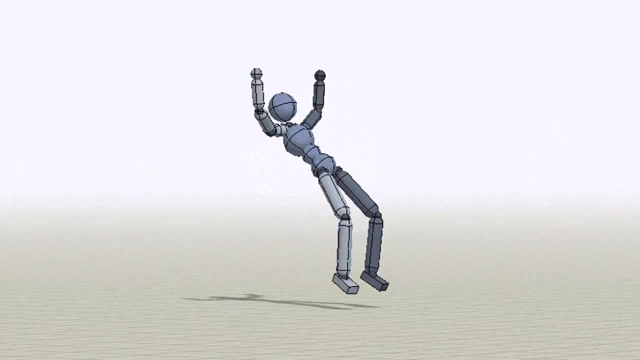 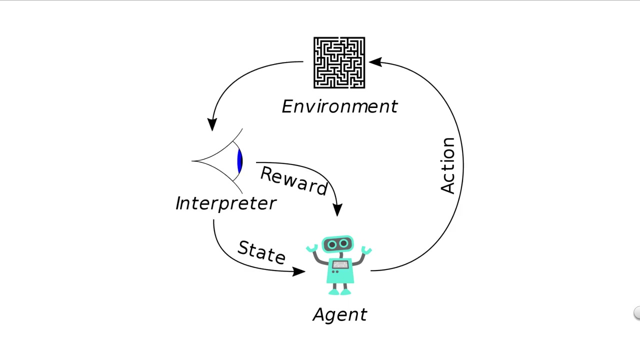 even teaching robots to backflip reinforcement learning is all based around a reward, and that brings us right back to q learning. q learning is one way in which agents, which are our ai programs, can attempt to maximize their reward. the idea is that if you can predict the reward from performing, 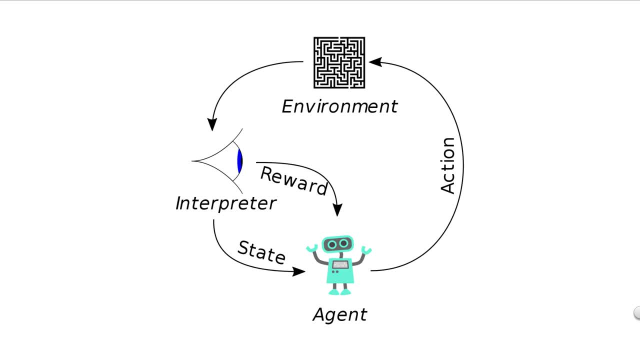 a number of actions. then you can keep choosing the actions that will yield the highest reward and, in the long run, get your desired goal. q learning is based on the idea of q values, which are estimations of the current and future reward your agent expects to receive. we can 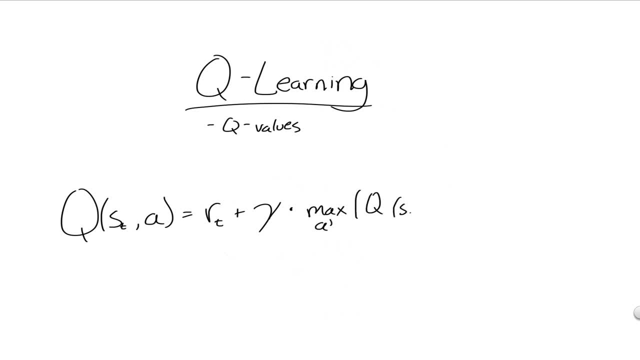 actually write this out in an equation to specify this, and it looks a little bit like this. now it may look complicated, but it's actually super simple. here you can see that the q value can actually be broken down into two parts: the reward from the current time step and a discounted 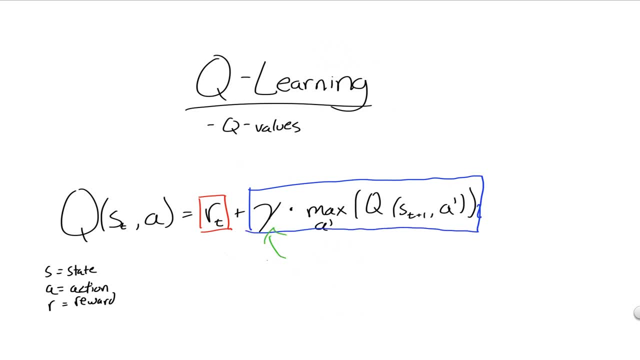 expense. here you can see that the q value can actually be broken down into two parts: the reward from the current time step and a discounted expense expected reward from future time steps. And when I say discounted, I mean we multiply this part by a number that indicates how important future rewards are compared to current rewards. So a 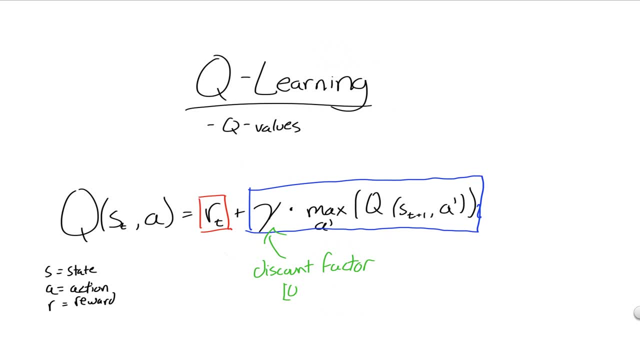 value of zero would mean we only value the current moment, while a value of one would mean we value the future just as much as the current moment, and we can use any value in between. So let's look at an actual example of tic-tac-toe. How would we approach this? Well, first we want to create a 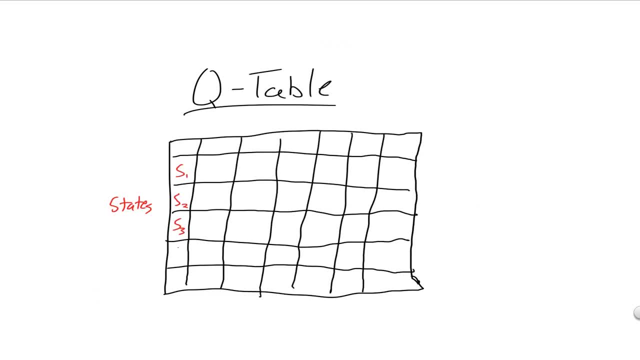 table, And this table maps our states of the game and actions into actual rewards, or rather expected rewards. Next we set the rules. So these are the default rules of tic-tac-toe. but if we win we get a reward of positive one for that final time step. But if we lose, 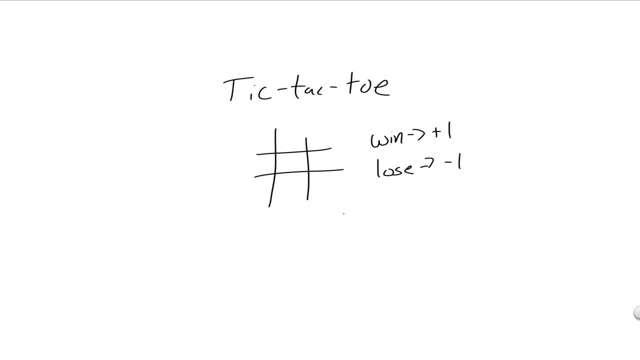 we get a reward of negative one, And at every other point when we make an action we just get a reward of zero. So let's say we play out a match And at first all the Q values are the same. So we 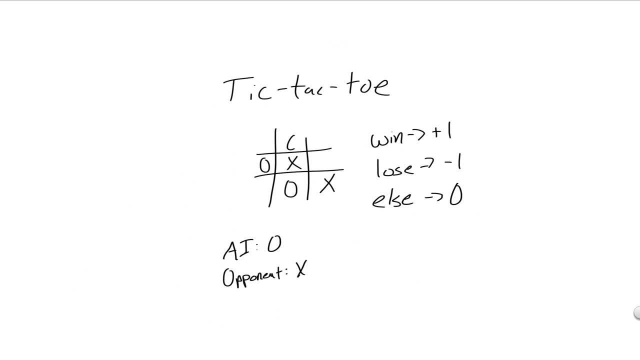 just choose actions randomly And, as you might guess, we end up losing. That gets us a reward of negative one, And now that we have received this reward, we go to update our Q table. Now, when we have another match and the opponent tries to pull the same move on us, we know not to. 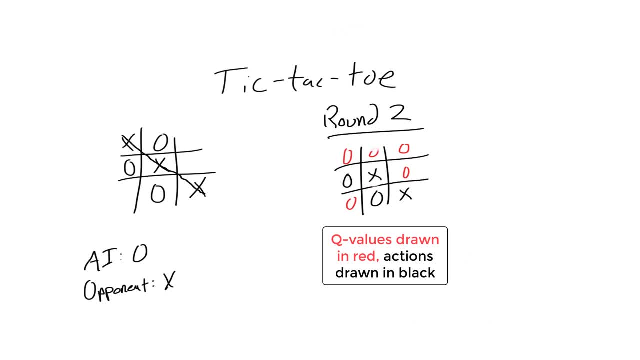 make the same mistake again. This process would continue on and on until we fill up our Q table, And then we should really start to play out our Q table, And then we should really start to play out our Q table, And then we should really start to play out our Q table, And then we should really